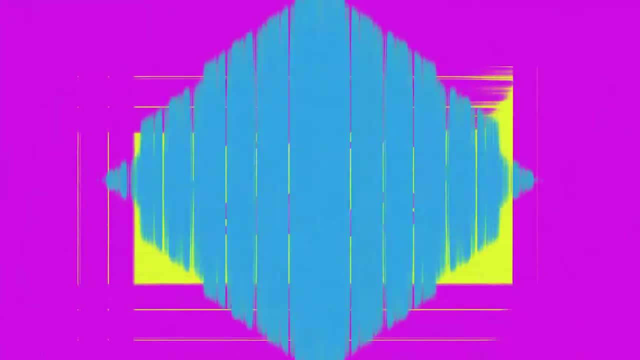 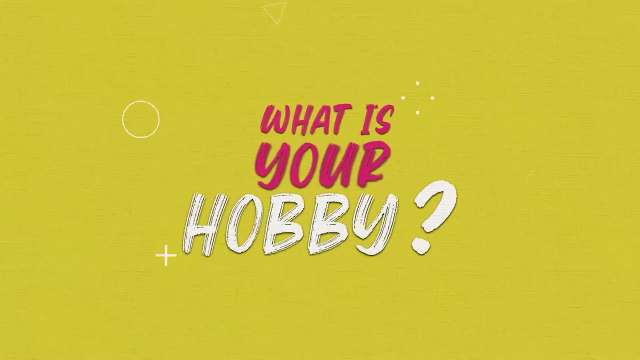 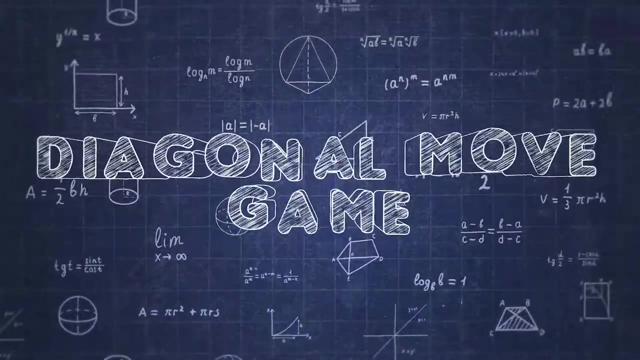 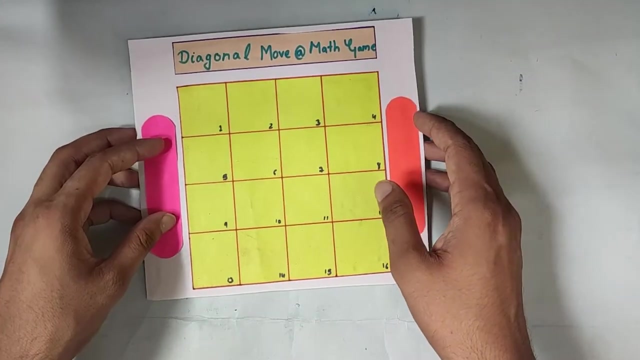 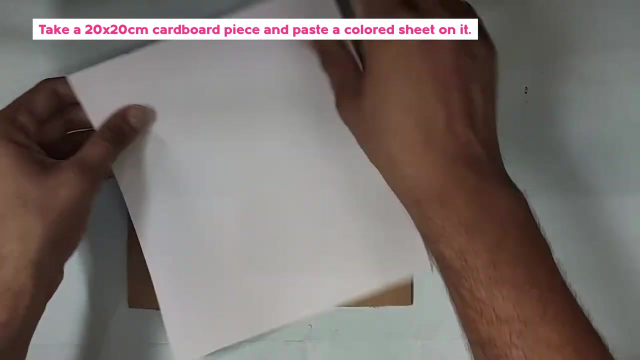 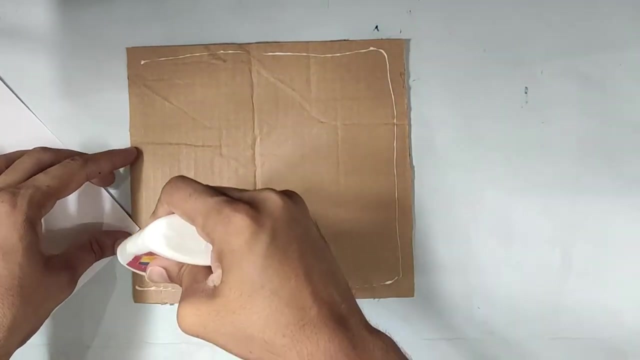 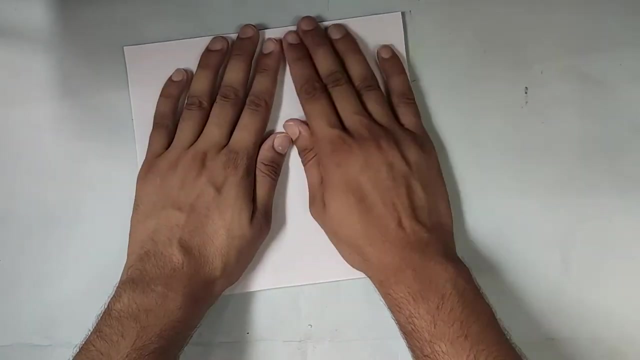 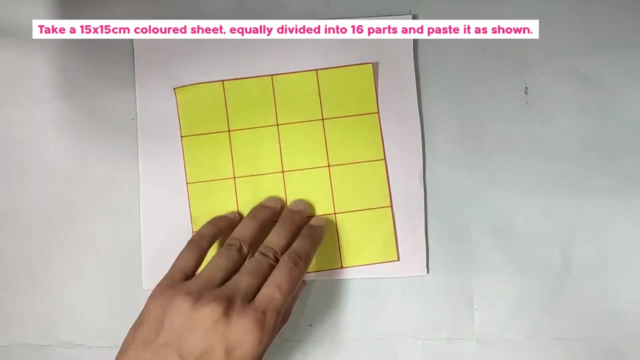 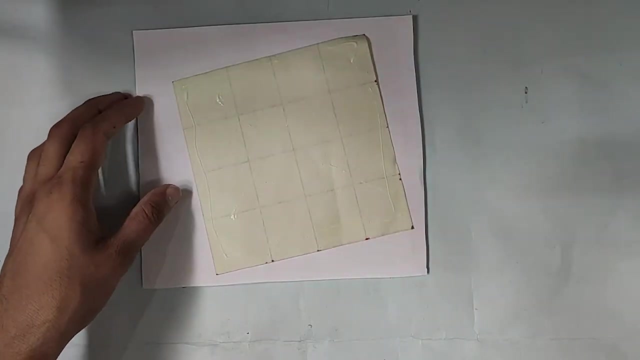 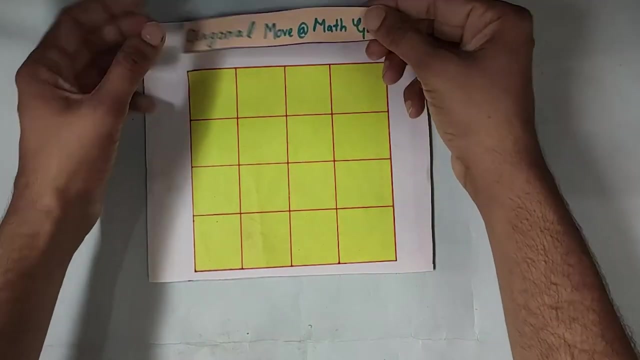 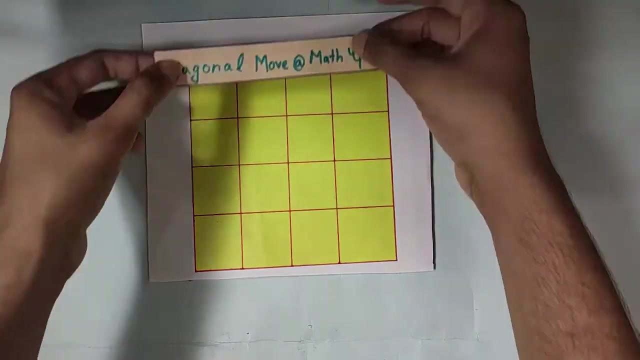 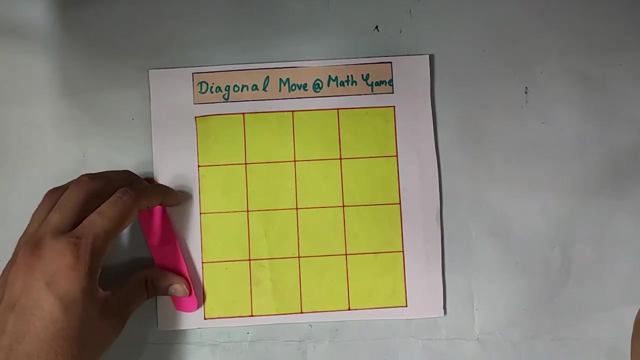 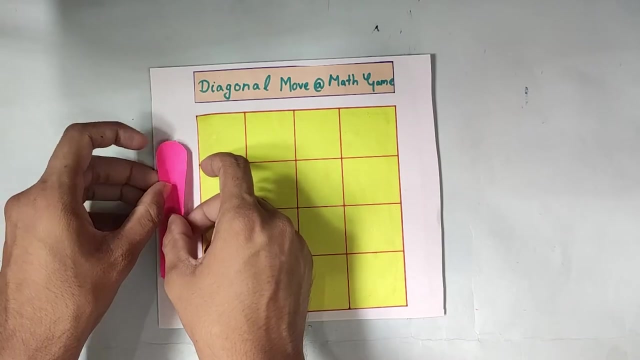 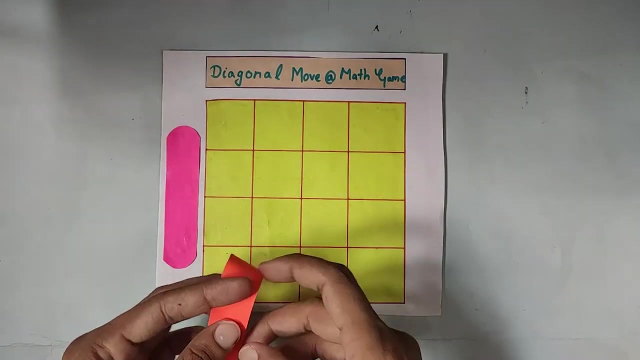 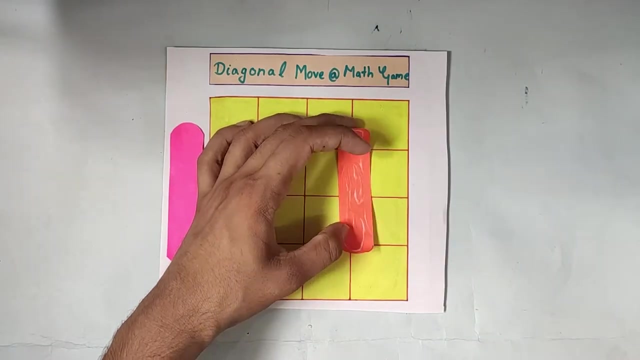 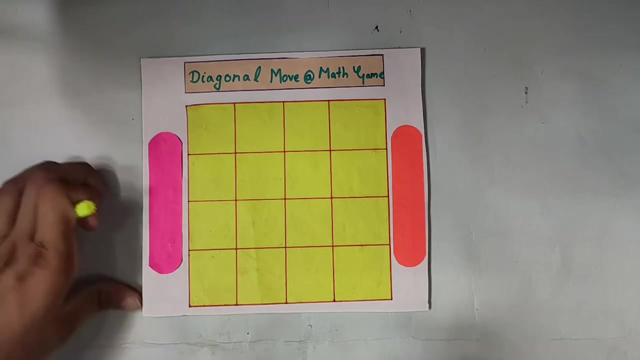 Hello everyone, welcome to another video of what's your hobby. In today's video, we are going to learn how to play a diagonal move game. We are going to learn how to play a diagonal move game. We are going to learn how to play a diagonal move game. 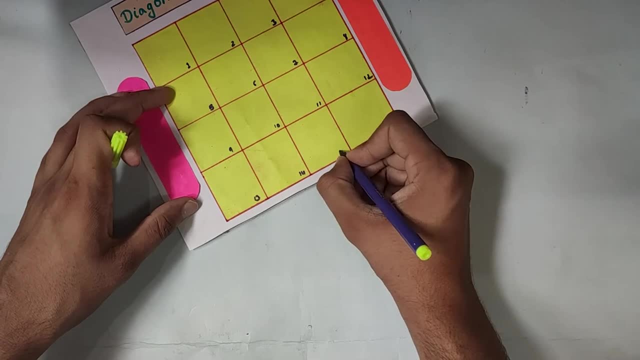 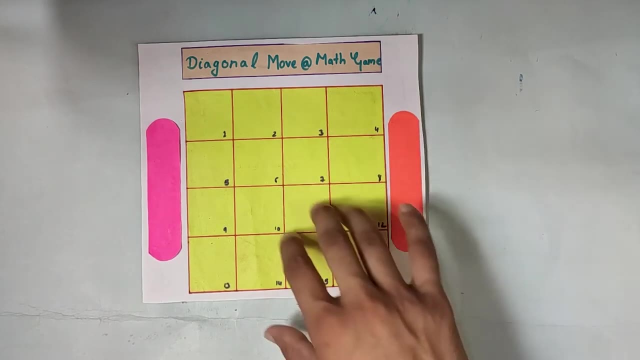 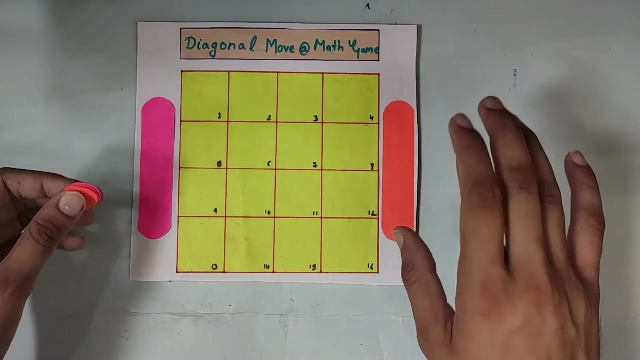 Now, as you have built this game. so let's quickly learn what are the rules of this game and what are the other things that you need to play this game Now. to play this game, you need four orange circles and four pink circles, and you have. 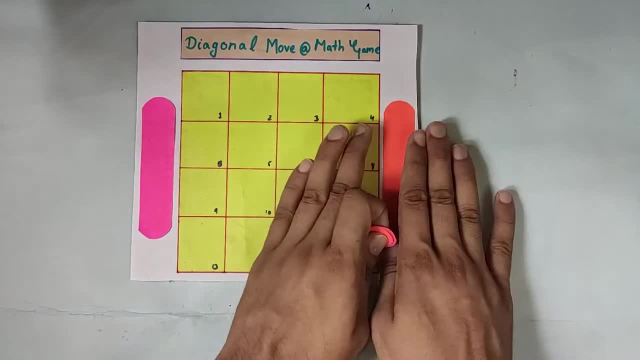 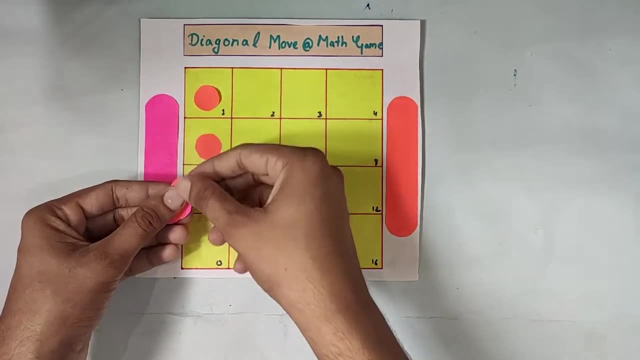 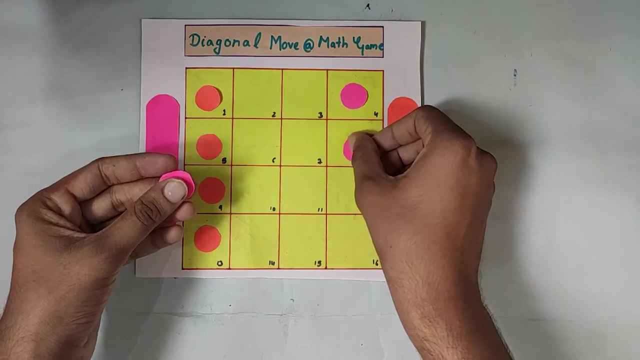 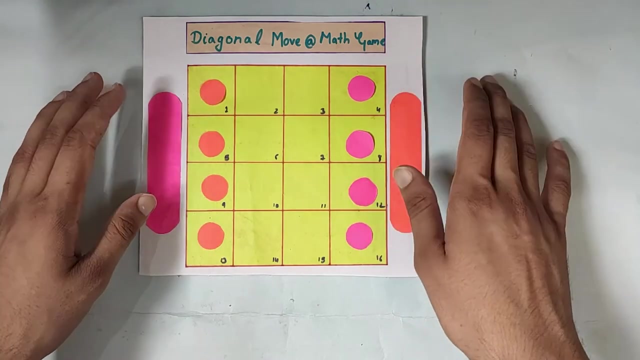 to place them in such a manner that the orange circles are opposite to this orange strip. You have to place them in this manner. The orange circles should be here and the pink circles should be here. The rules and the winning condition of this game is quite simple. 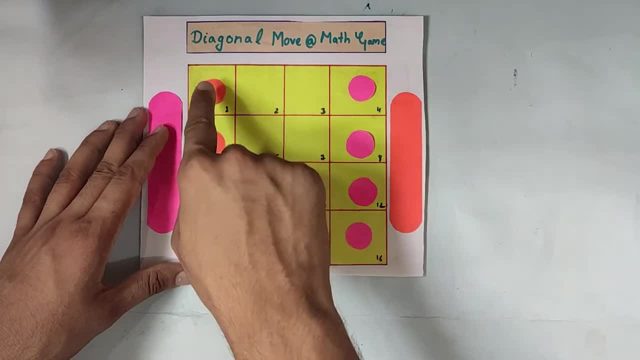 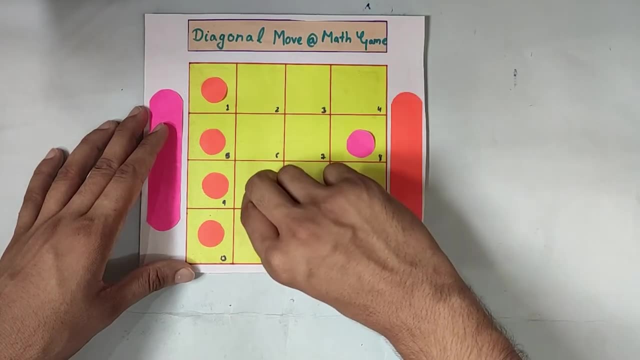 The winning condition is that you have to take these pink circles to this side and these orange circles to this side, But you can only move these circles diagonally. Now let's see how to play a diagonal move game. First of all, you have to move these orange circles to this side and these pink circles. 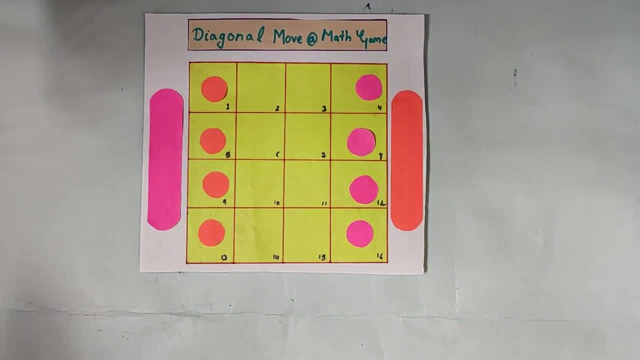 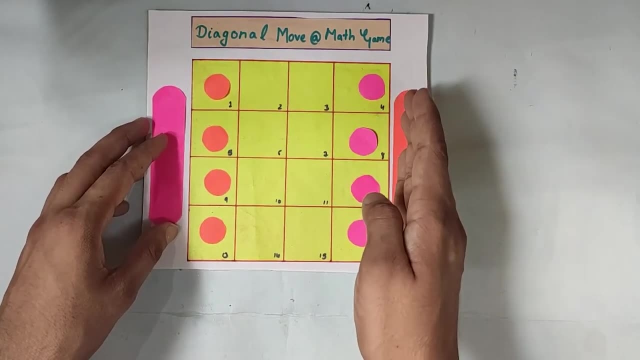 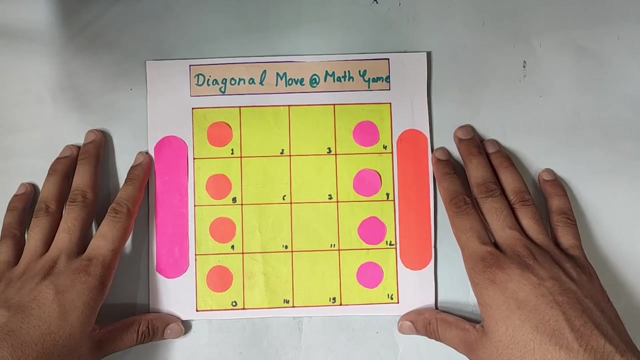 to this side. So the game looks quite simple, right, But actually it's not. The condition is that you need to move these pink circles to here and these pink circles to here only in 14 steps. Let's quickly take one example on how we can play this game. 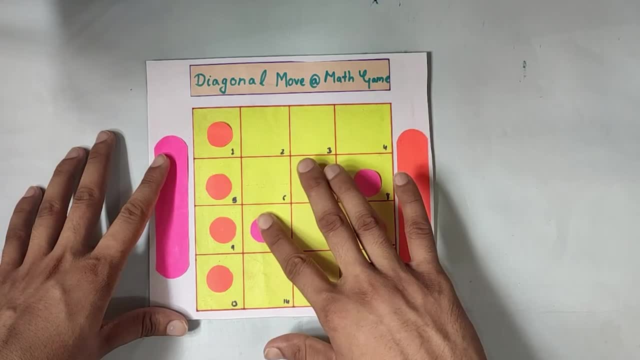 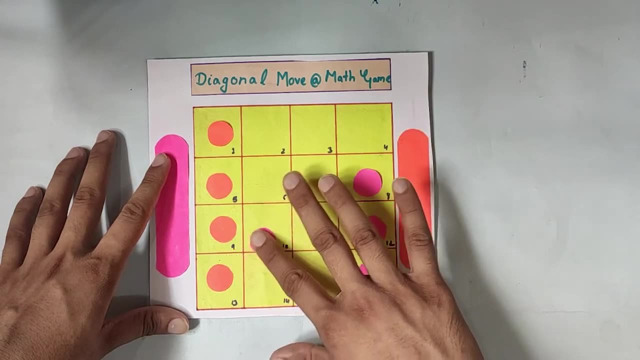 So let me start with this. So this is one move. either you can move two at a side or just here. This is called one diagonal move, either to here or to here, or to here as well. This is one diagonal move. 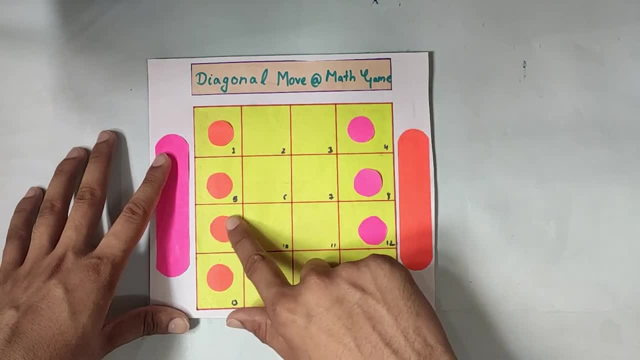 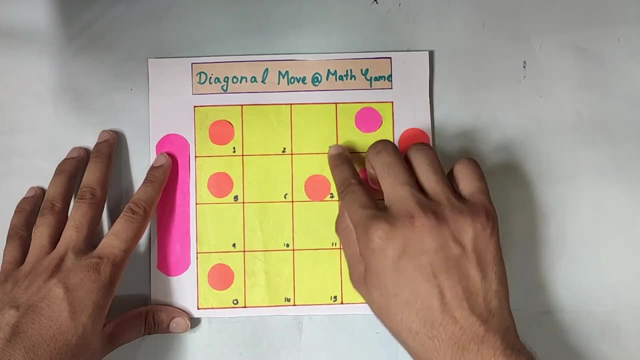 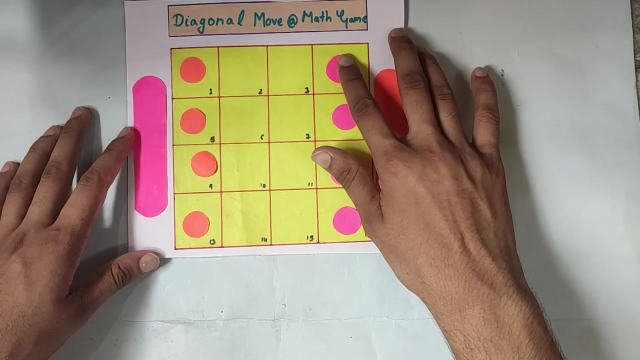 One more rule is that you cannot jump over another circle. For example, if the circle is here, you cannot move this pink circle to here. This is not possible. Let's quickly take one example on how to play this game. For example, I move this pink circle to here. 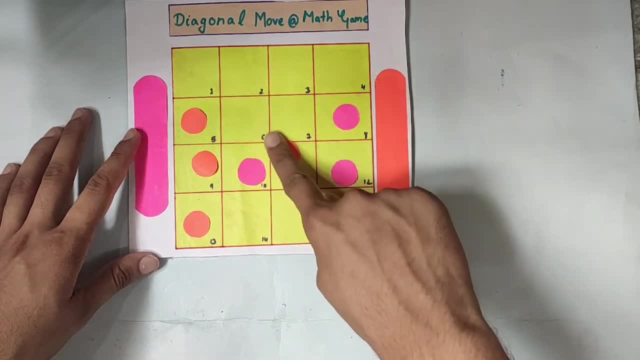 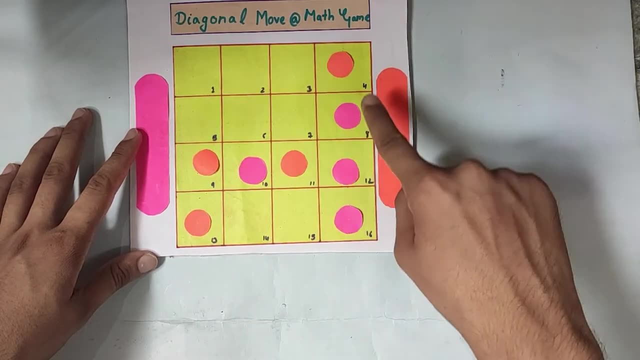 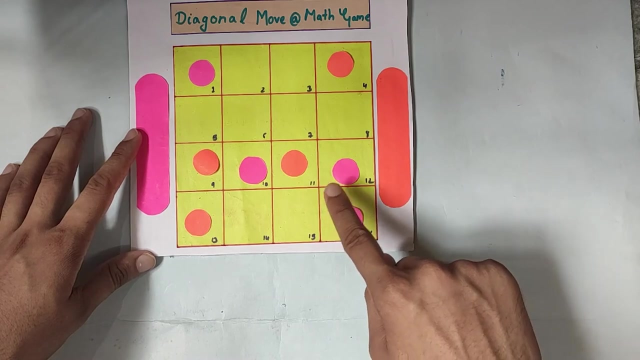 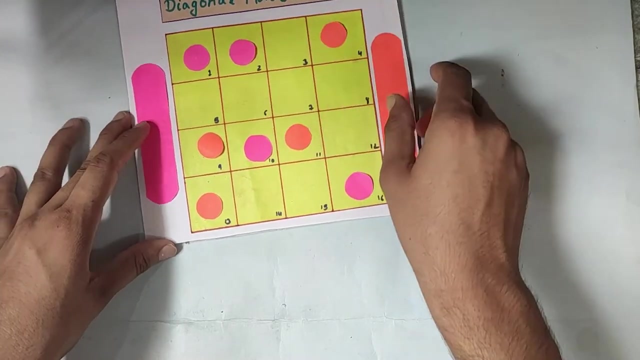 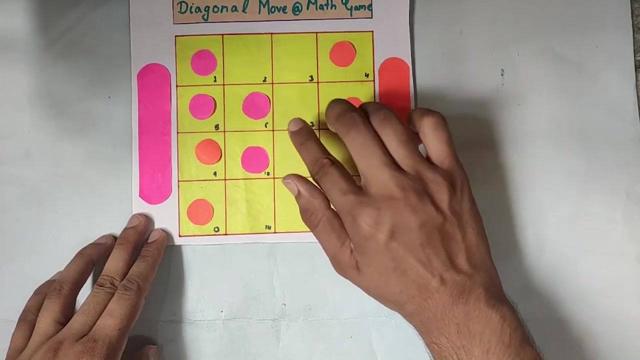 It's one step. Now I move this orange circle to here. It's two steps. Now it's three steps, Four steps and five steps. Similarly, it's six steps, seven steps and eight steps. okay, Now let's move this ninth step to here, and it's 10 steps: 11,, 12,, 13 and 14, 14 steps. 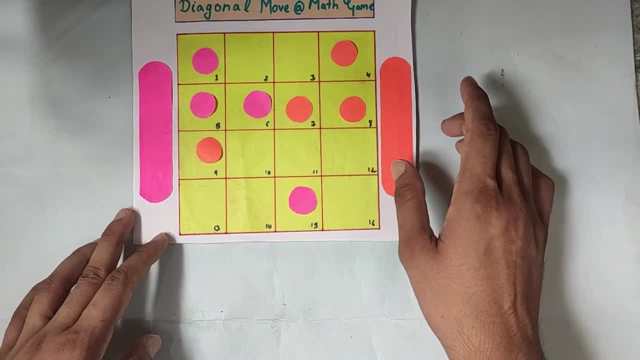 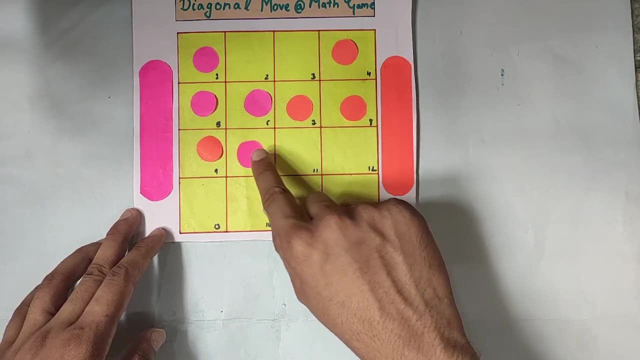 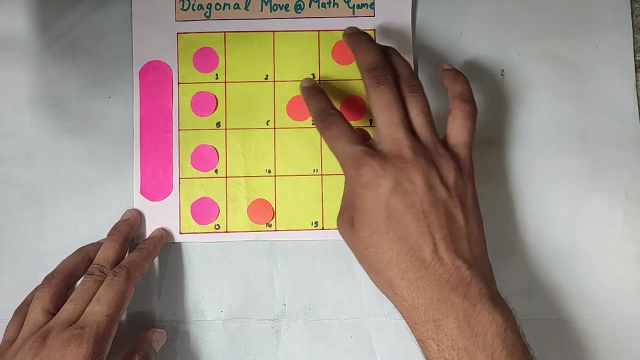 are over, But still the game is not complete. We will continue till when it goes like the steps. 14 are over Now: 15,, 16,, 17,, 18,, 19,, 20 and 21.. So the game is completed in 21 steps. 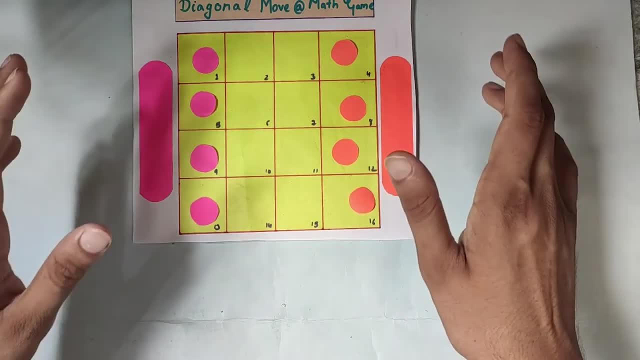 But that is not our aim. Our aim is to complete in 14 steps. As the game is not completed in 14 steps, we will continue till when it goes like the steps. 14 are over. 11 steps are completed in 14 steps.